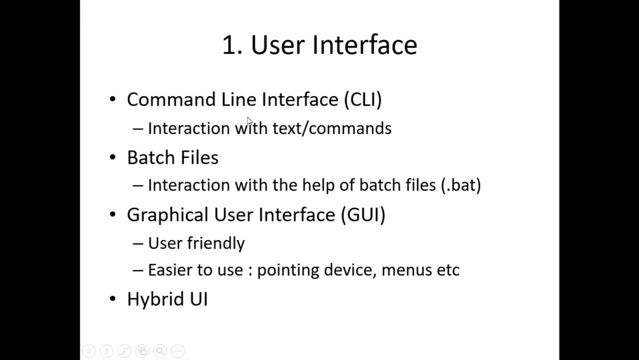 command line interface. so in this user interface the user is expected to enter in or like key in, the commands using some like using the keyboard, and then execute the commands. basically so user would be like expected to enter in all the commands and then send it to the operating system to handle those. 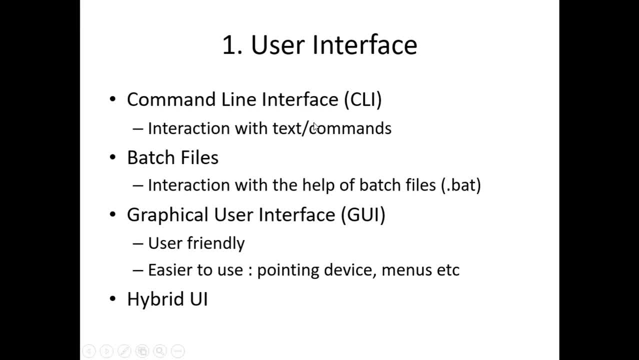 commands. so here interaction is basically with text or commands. and the next, next type of UI is basically this batch file based. so when we say batch file based user interface, it is kind of similar to CLI, but the only difference is that instead of directly executing commands, we execute the batch file. so 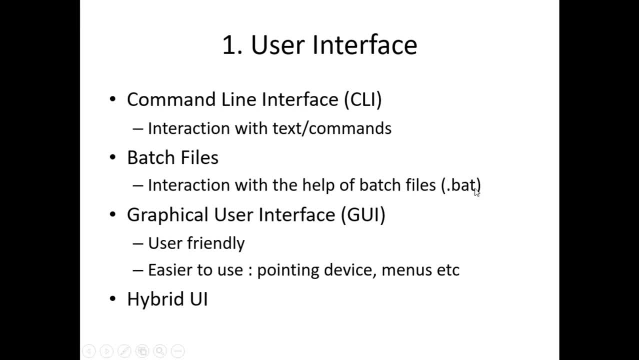 batch files are those files which have this dot bat extension. so a batch file is nothing but a file in which we have, like, a series of commands and when executed, all the commands are like, executed sequentially, so line-by-line, all the commands will be executed and operating system will continue executing until they're like. 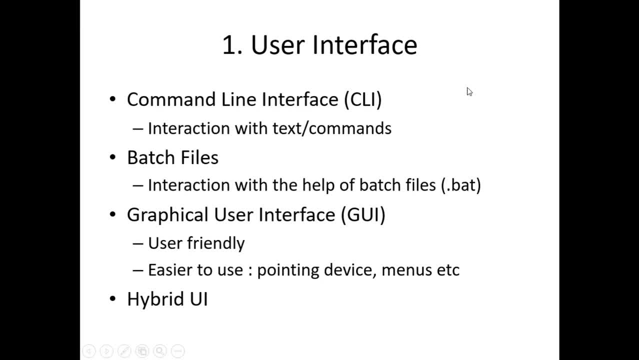 there are no no more commands left or operating system can also like stop executing, if at all. there is some error in one of the like intermediate commands in the batch file, that is, batch file based UI, and the third one is the most popular one, which is the JPEG file based UI, and the third one is the most popular one, which is the. 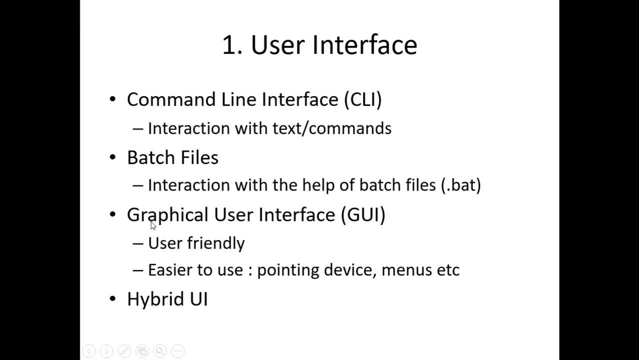 GUI- graphical user interface. this is like more user friendly, because it allows users to interact with the operating system with the help of pointing devices like these mouses, and we also have like menus and all. so using GUI also, it is possible to interact with the operating system. so these are some of 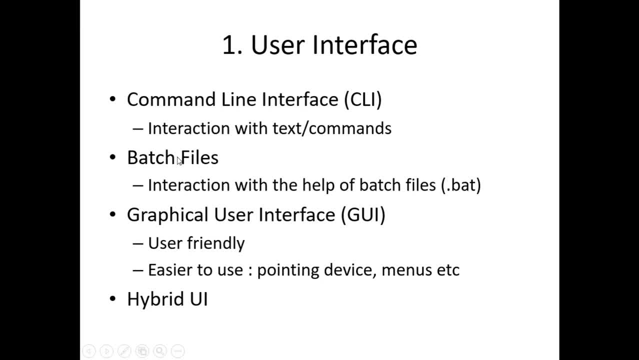 the like major types of UI which are provided. apart from this, there are cases where operating systems provide a hybrid UI. by hybrid we mean that it has a hybrid of both the GUI as well as CLI, so it would be mostly GUI. buthei would be provided as a special program which the 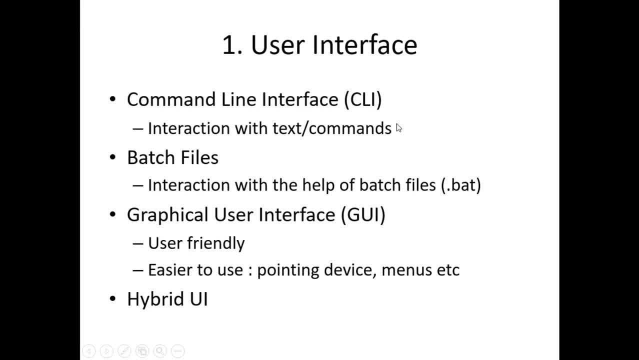 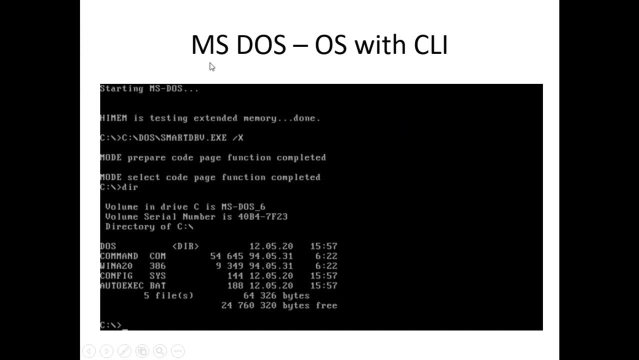 user would have to like run in order to like run this year CLI. so here is an example of an operating system which has CLA as its UI. This is MS-DOS, if you see here a user would have to like enter in the command. so these are some of the 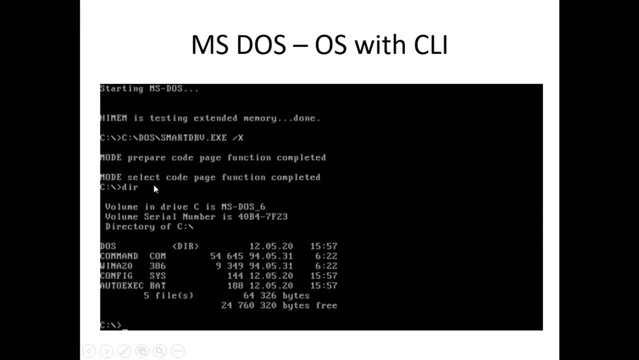 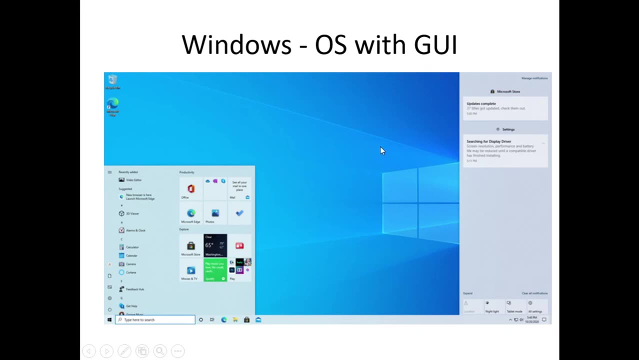 commands which user is entering. for example, there's directory command. user will enter and always will like provide all the list of like directories or like files. and the next type is like Windows, which is like an OS with graphical user interface. so here, if you see, we have like my nose, and it also provides these. 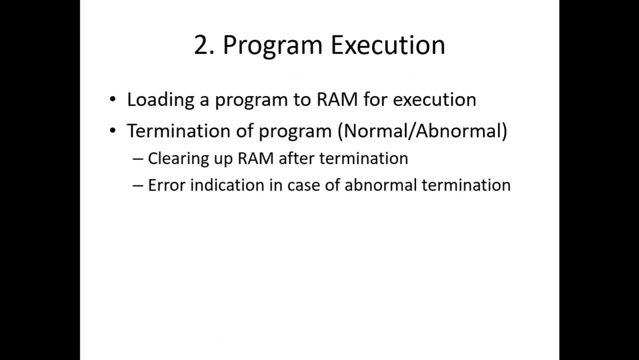 pointing devices and all so when they come to the next like service which is provided by operating system, is this program execution. so whenever when we say program execution, it is nothing but loading the program to RAM for execution. so it is the operating system which handles this program execution. and 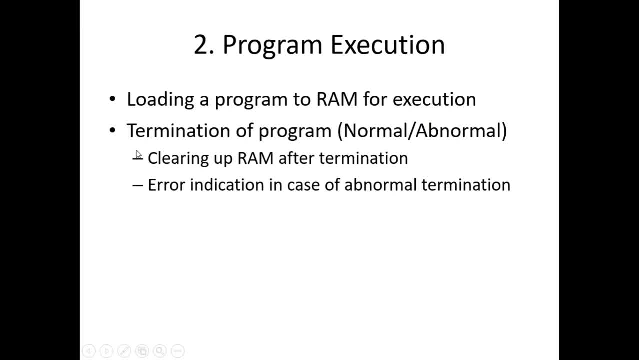 apart from program execution, the termination of program is also handled by operating system. so assuming the termination is like normal, then in that case whatever program was loaded to RAM should should be like cleared from RAM, and in case of abnormal termination, operating system would just like show some kind of error code and then 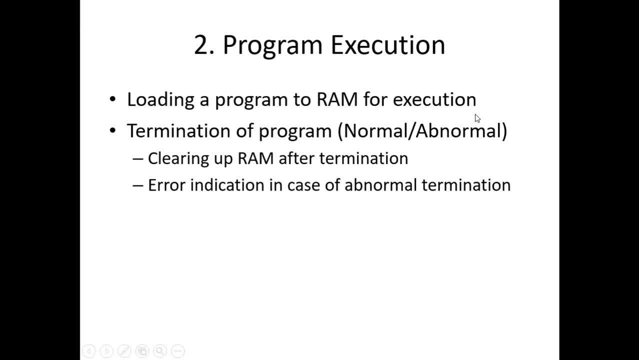 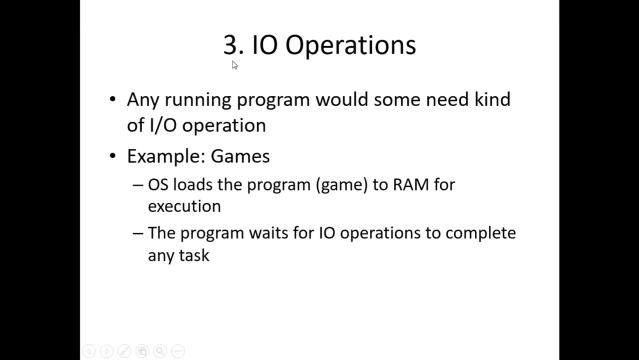 it's just like do some abnormal termination. so whenever we just like click on some application in the background, it is the operating system which loads the program to RAM and then executes it. so that is regarding this program execution. and when we talk about the third service which is provided by 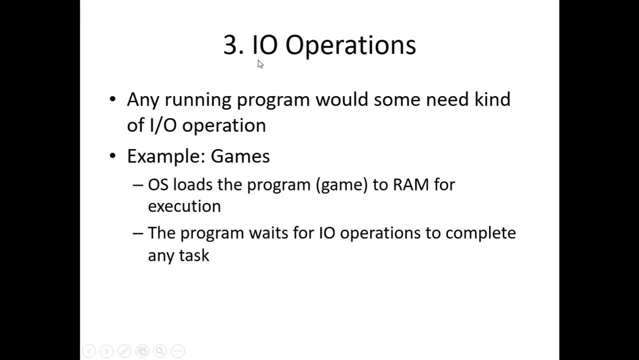 operating system. it is the IO operations. so whenever we run any program it would basically need some kind of IO operations to be performed in it. so, for example, if we are running a game, so we'll just like double click on a game and operating system will load that game to RAM for execution and this game would 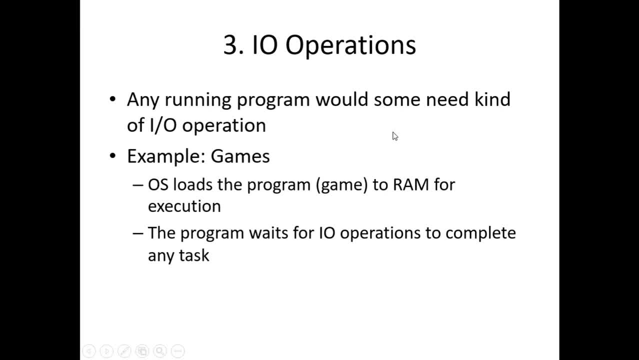 start, but it would actually wait for some kind of IO operations to like proceed. for example, if you want to like open up settings, then you'll have to like type in- I mean use your keyboards or like mouse or something- and that handling of IO operations is again made possible by operating systems. the fourth: 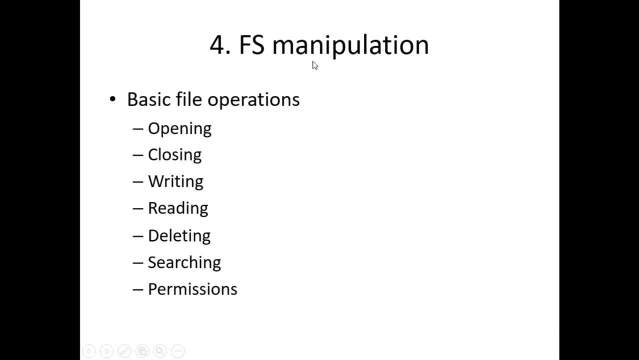 one is the file system manipulation. so it is the operating system which helps in providing the various file operations, like, for example, whenever you open the file, it is the operating system which is working in the background to open it, and similarly, when you are closing it, whenever you. 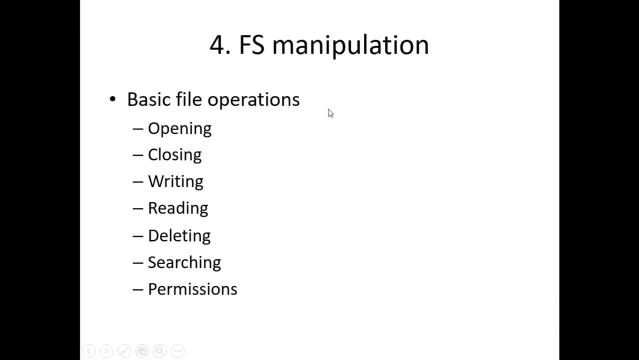 write it. so it is the operating system which handles all the writing part, reading part and also saving it whenever you delete it. it is the operating system which is like helping in deleting, like the file tighten or opening a file. in a way the file does not continue to openığım. 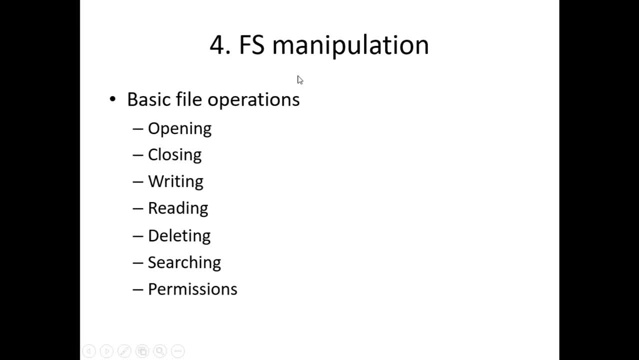 and also searching the files. and also operating system provides various permissions for files so that some users only can access some kind of files. so there are like restrictions, which are also possible to be like provided using operating systems. so these are some of the basic file operations. there are like: 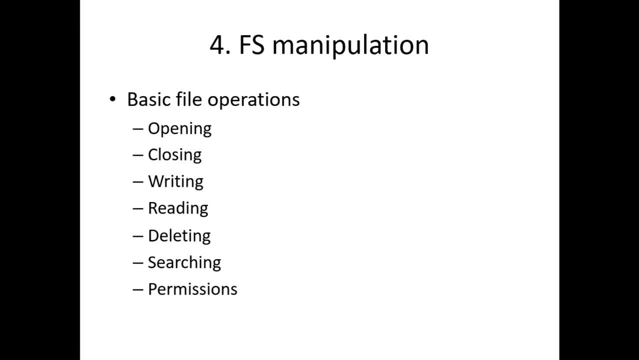 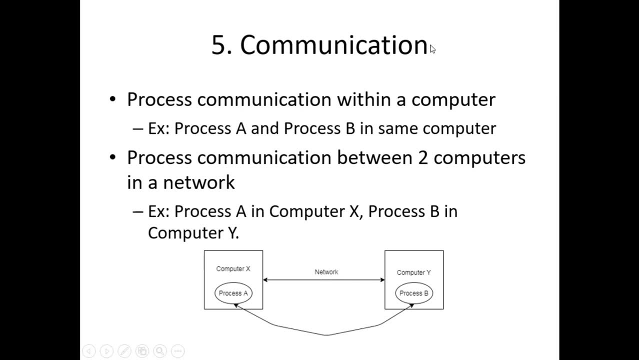 many other file operations also which are provided by these OS's. the fifth, fifth type of service is this communication. so when we say communication it is nothing but the communication between processes. so here two processes within one single computer may need to have like some kind of communication between them. that would also be like made possible by operating. 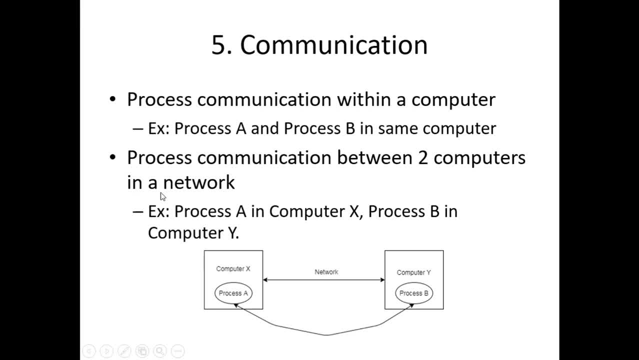 system. so operating system will try to like set up this communication between the two processes. and apart from that there might be cases where two computers are connected like with some kind of network and process. one process in some computer would might want to like a communicate with some other process with like in in. 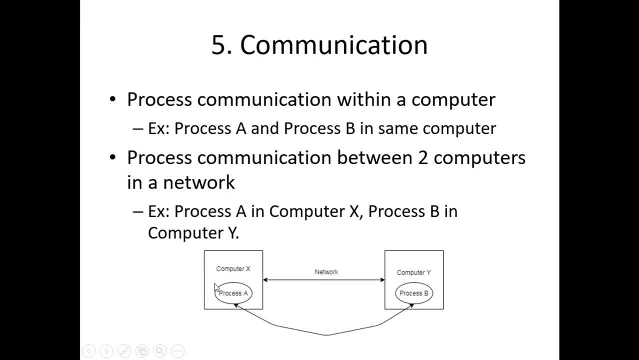 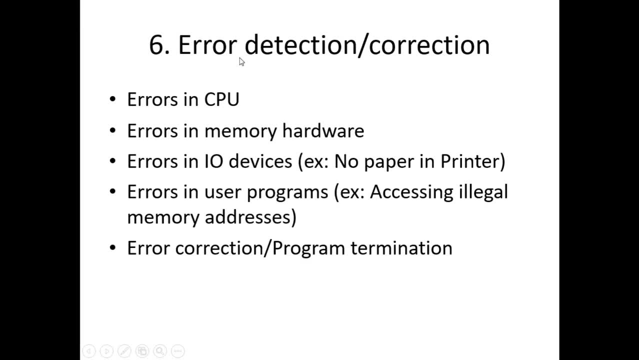 some other computers. so there also this process, communication is made possible by the operating systems in these two computers. the sixth service is it talks about error detection and correction. so when we say error detection these could be like errors which are there in CPU or in like memory. 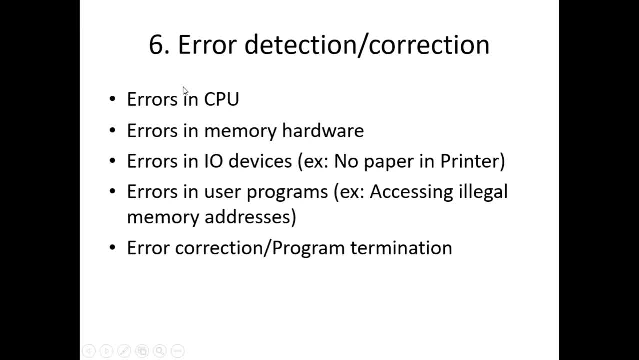 hardware, say there was some kind of power loss, so operating system should be able to like handle that, and there might be errors in IO devices. if we consider a printer as an IO device, error for example could be like there is no paper in the printer, or also we might have like errors in the user programs itself, like for example, 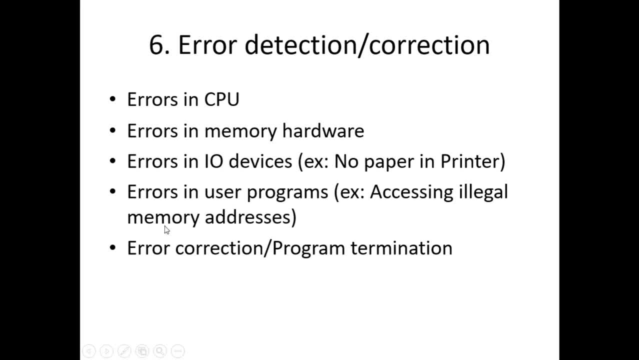 there might be certain like memory addresses which are illegal to access. so if at all a user is like accessing those illegal memory addresses, you always will detect that error and try to give the error code to the user saying that the user program is trying to access illegal memory address or something like. 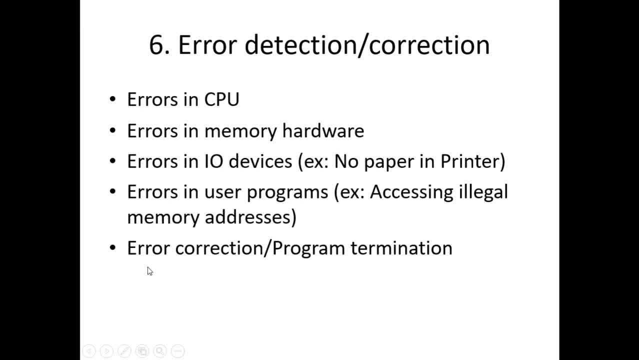 that, and apart from that, there might be cases where operating system itself tries to correct the errors by like terminating the program, or if at all termination is not possible, then it operating system might like abruptly stop all the programs which are running, or it can like restart the computer. 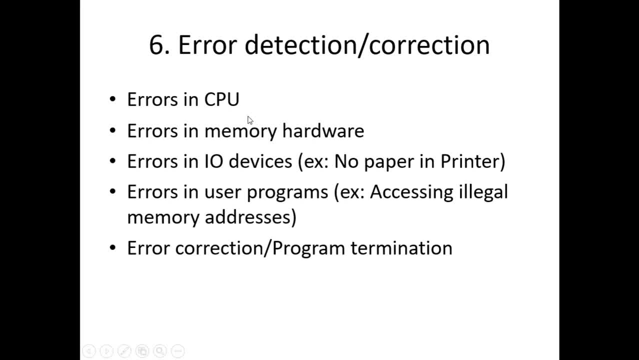 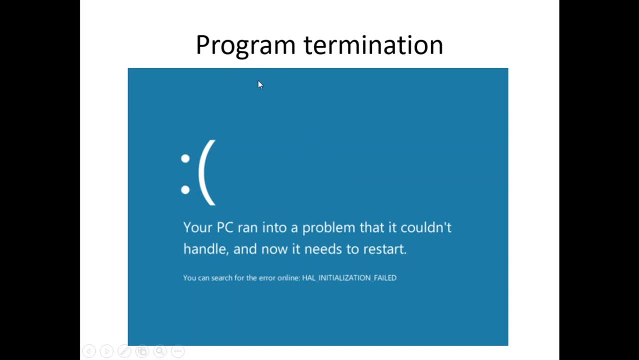 or whatever. so those are the error detection and correction mechanisms which are like provided by operating systems like, for example. this is one of the ways in which operating system handles some kind of error. so if at all there was some problem, and if operating system wasn't able to handle it, it will. 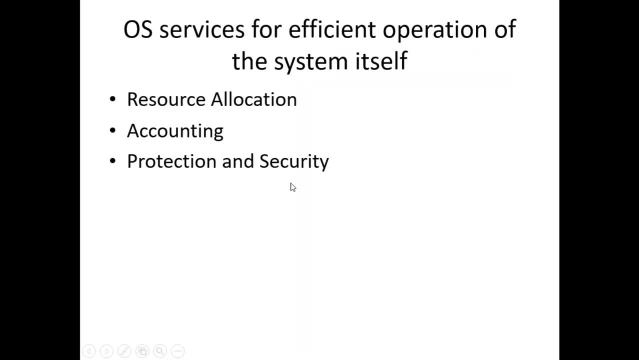 just restart the computer. so those were some of the operating system services which are provided for the users, especially the users themselves, and there are some more group, I mean there are some more types of services which are meant for having, like, an efficient operation of the system itself. so here we talk about resource allocation and then operating. 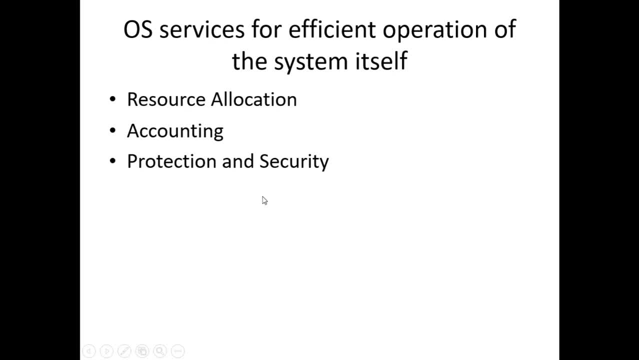 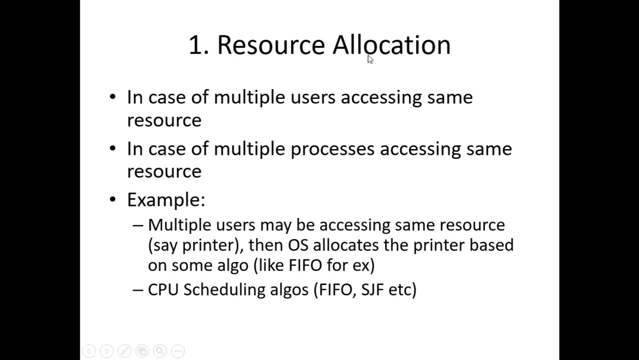 system also maintains some kind of accounting. it also provides protection and security. so we'll go over each of these points in detail now. when we talk about resource allocation, this usually comes to picture when we talk about cases where multiple users are accessing same resource, for example, assuming there is like a printer and one printer is being accessed by, say, 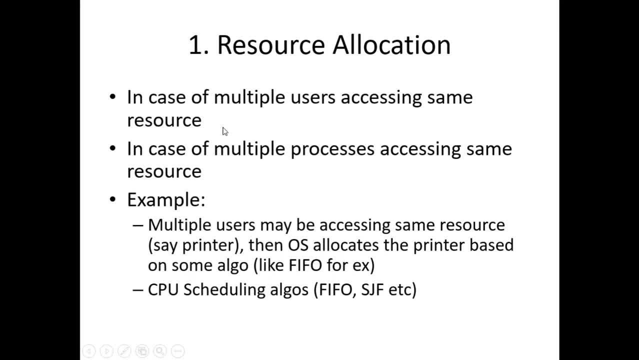 like five or six users and if at all like all of those users want to like print at the same time, then operating system would have to handle all the requests in some kind of way. for example, it may use this first-in-first-out algorithm or some kind of algorithm to like provide this resource to all the 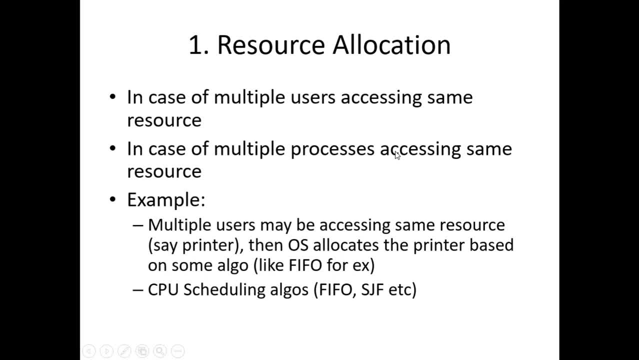 users. apart from this, there might be cases where multiple processes are accessing the same resource at the same time. in that case also, operating system may use some kind of algorithm, like, for example, they have these CPU scheduling algorithms like shortest job first or FIFO, etc. so it just like picks up one of 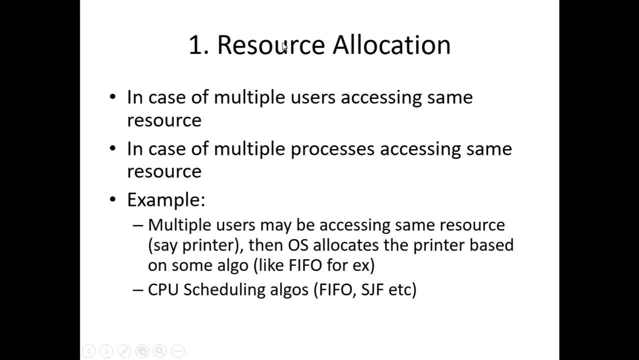 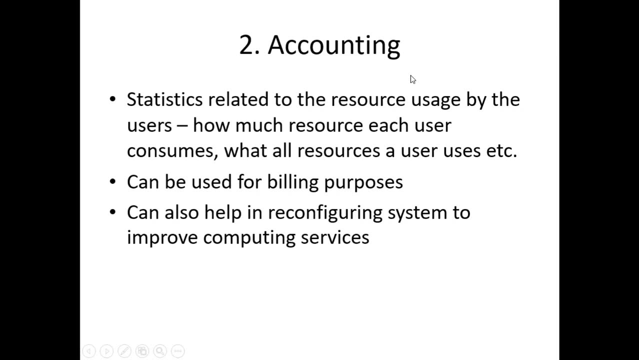 the algorithms which is like most suitable. and then it tries to provide resource to all these processes which are trying to request for resource, so that job is again handled by operating system. and apart from that, there might be like some kind of statistics which are related to the use, usage of resources by the users, like for example, how much 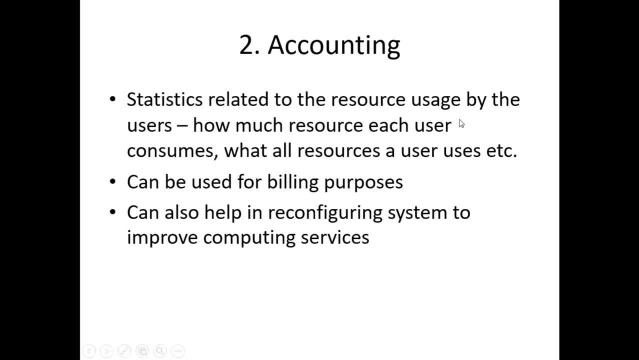 amount of resource one user is using or what all resources a user is using. so all those statistics are also maintained by operating systems. so this stats can be like used for billing purposes, or may also be used to like reconfigure systems to try to improve the system. 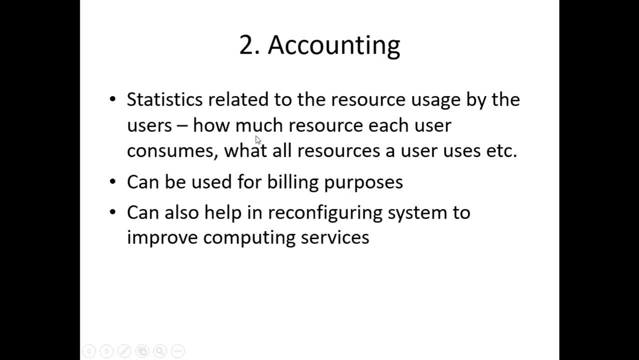 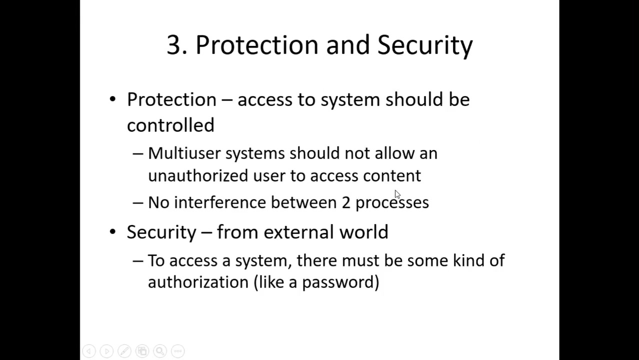 So when we know that some user is making use of, say, like some is abruptly using more amount of resources, then in that case we can try to reconfigure the system. or if, if at all, a user is using multiple resources, then it can be like used for billing purposes also here. the third: 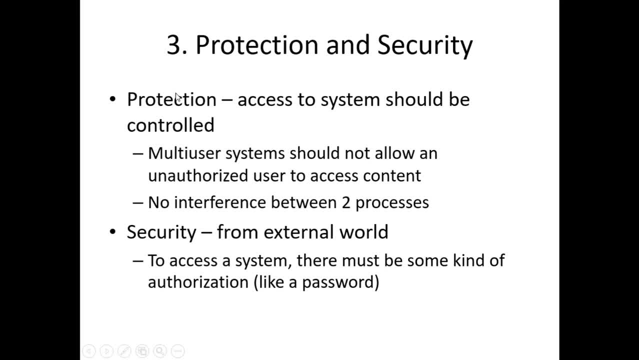 thing is about protection and security. so when we say protection, it's it is nothing but access given like access to the system should be like controlled here. so when we say access to system, we we are basically talking about multiple users using the same system. so here, if you have a multi-user system, 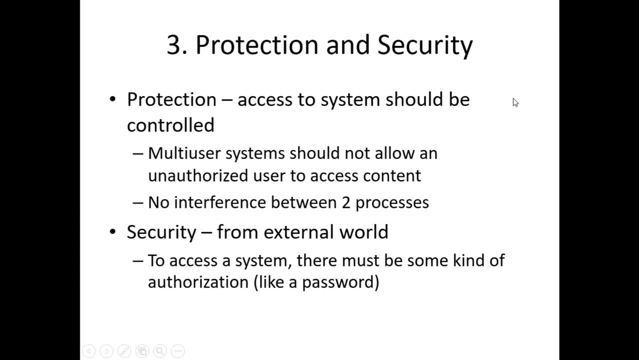 there there might be, like certain content, which is authorized only for certain users and any unauthorized users aren't allowed to access the unauthorized content. so basically that kind of protection is provided by operating system. apart from that, operating system also makes sure that there is no interference between two processes or between a process and 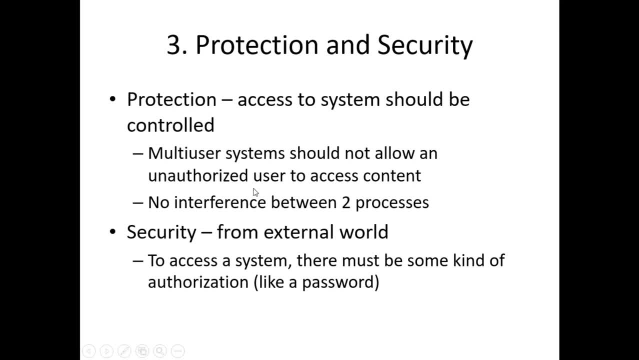 even the operating system itself. so that kind of protection mechanism is provided by operating system and apart from that we also have security. so when we say security, it is basically the security from the outsiders. so in order to access a system, the user should be able to like show that he has the authorization. so the most basic example.